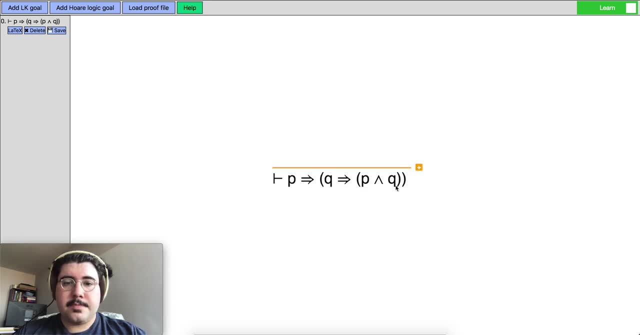 So suppose you want to prove this. So this is an incomplete proof tree. So this is an incomplete proof tree. We start from the goal and you build upwards. but by clicking on the button plus, here you can see all the possible rules to apply, And here you want to apply the implies-right rule. 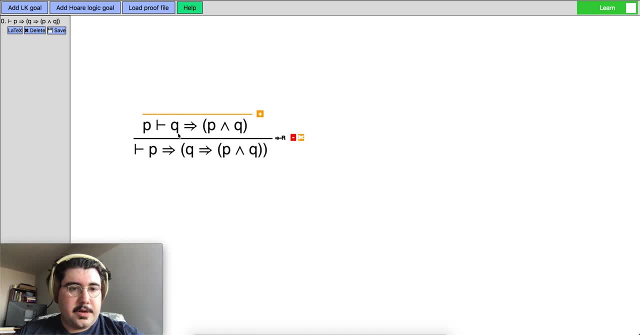 and we do, and it is applied, And we do, and it is applied. So here you want to apply And s'applies the implies right rule again, and we got that. and now we want to apply the end right, and it is applied. and these are just the identity rules. 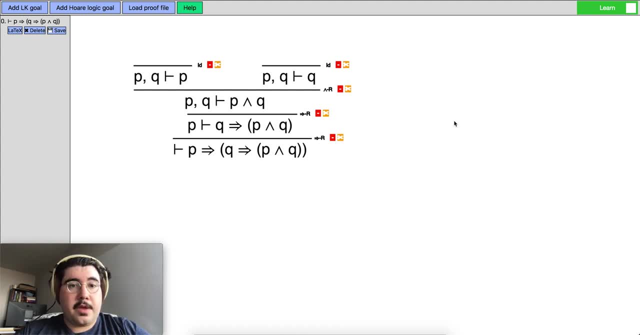 so this is simple secret calculus proof as it is done by the users. so this is sort of inspired by the whole driven development style of certain interactive theorem provers like agda or certain programming languages like Idris or Haskell. this idea goes back to mid 90s and another. 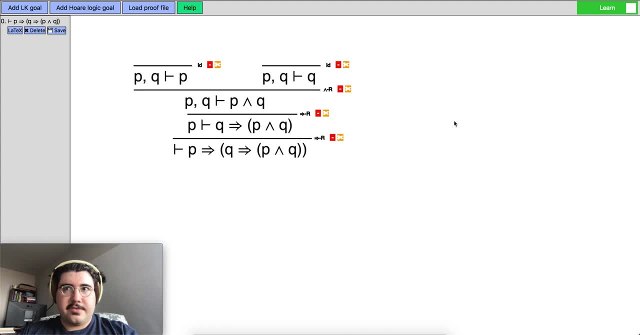 spring stream for this is, of course, structural editors, which go back to 70s and most 80s. so I wanted to create a proving experience that, based on proof trees, that imitates that, the usefulness of that. so what are the other buttons that you see here? 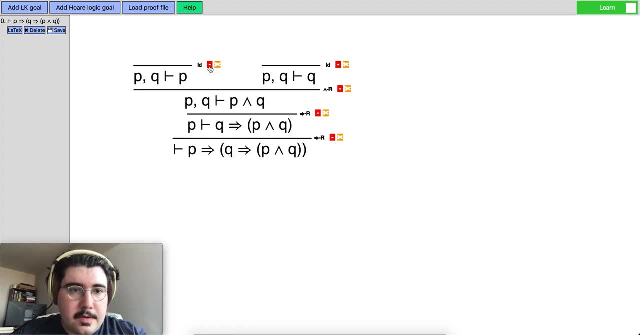 um, so so. so for each proof rule applied, you see two buttons. there's a minus button, there's a scissors button. so the minus button just unapplies everything that you did above that line. so if you made a mistake and if you want to go back and erase the applications of rules, that 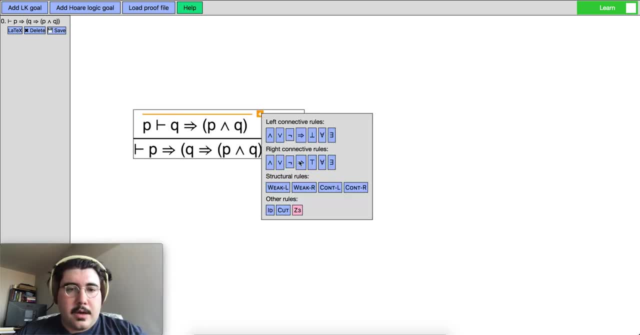 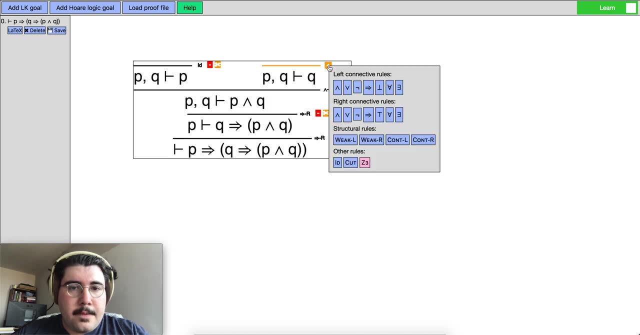 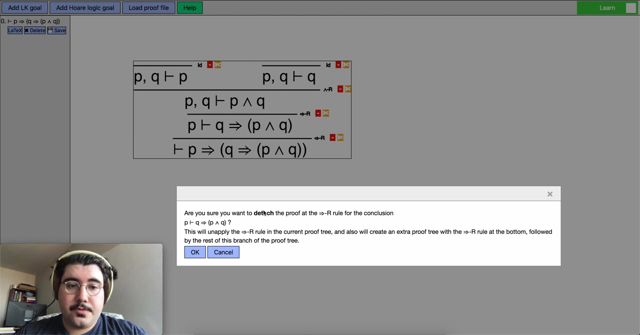 you have. it's a useful feature, so let's have some of these again, just to show. so the other button that we have, the scissors button, cuts the proof in half, uh, separatng from from that line. so I click on this and it's asks me if I want to detach the proof at this rule. 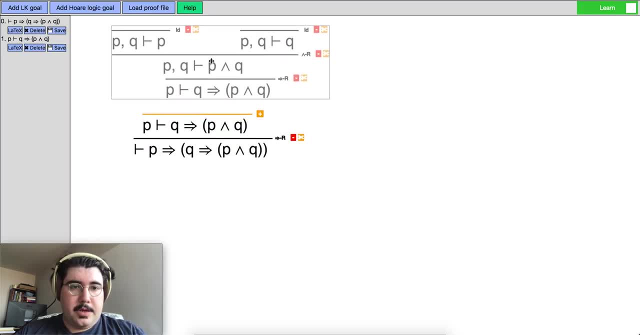 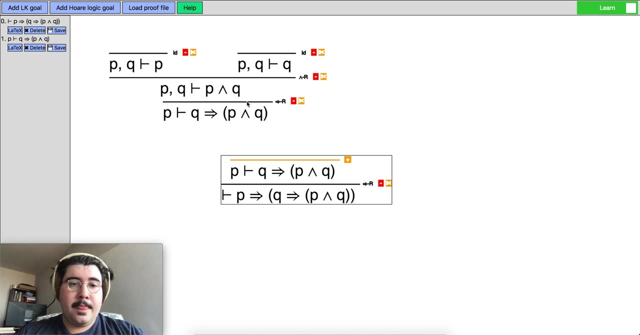 um, I do so. now we have we have two proof trees. this is the initial proofing 3 that we had and this is the part that we added later, and then we separate into two. so this is useful in super普 לע, and this is the part that we added later, and we separate it into two. 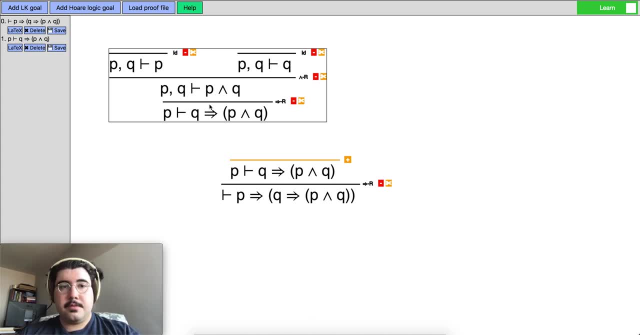 if certain people are proving something together and one person wants to prove one side of it and the person wants to prove the other side of it, And then they can combine these proof trees. So, as you see on the left side now, we have two proof trees listed here. 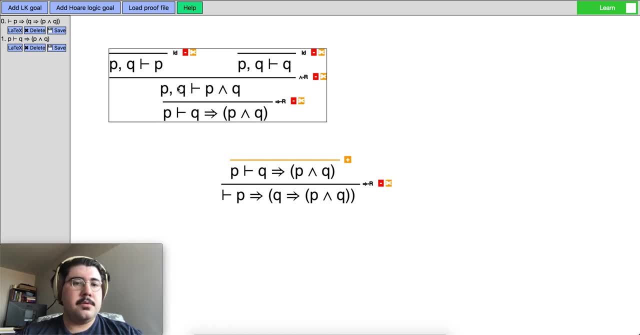 So using these, you can keep track of how many proof trees you have in the workspace, And to combine the proof trees you just drag the one on top and drop it on the other proof tree. Notice how, as I go in, the border of this goes yellow. 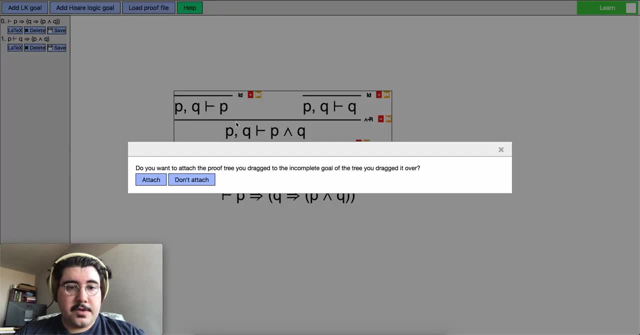 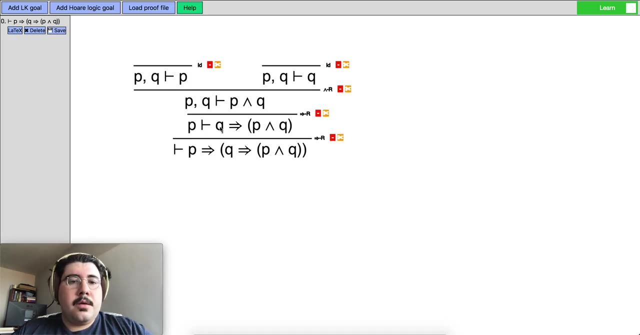 which means this is attachable again. So I do this and ask me if I want to attach, And I do want to attach. So now I'm back to where I started. So these are the sort of editing actions that you have with proof trees. 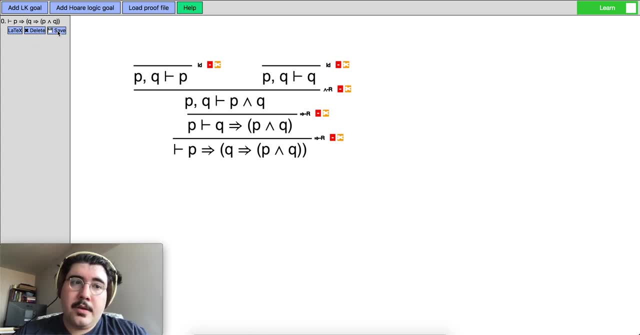 Also, you can delete entire proof tree. You can save it. There's a file And you can also copy the LaTeX output for this proof tree, the code that will render the LaTeX version of this proof tree In fact. let's try that. 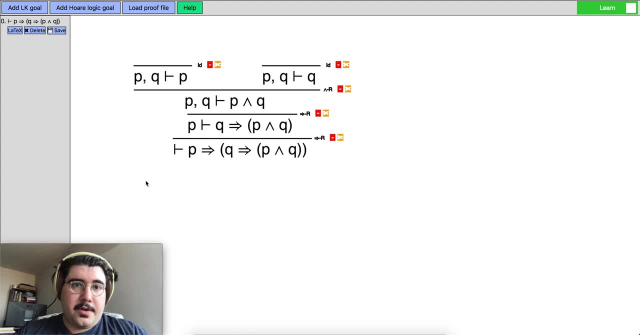 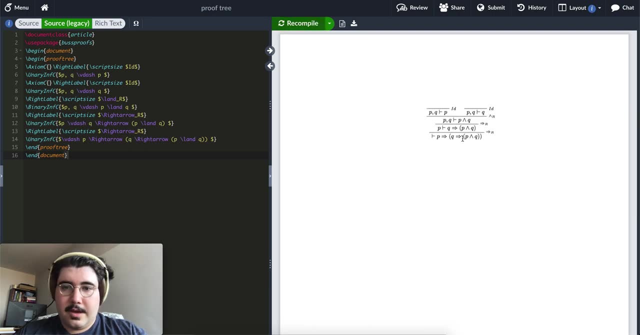 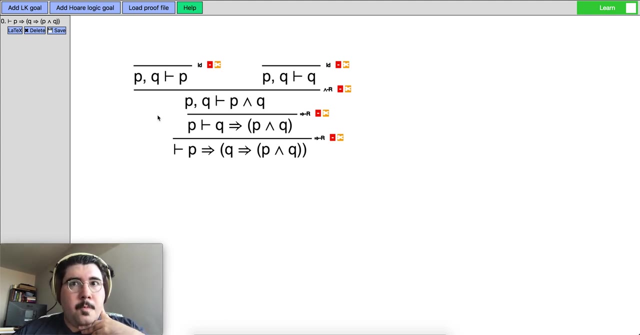 So I click on this, It is copied to my clipboard, And now, if I go to a LaTeX file and compile, I'll get the proof tree that I want. So what, what kind of edge cases do we have for this? So let's try that? or what kind of error messages? 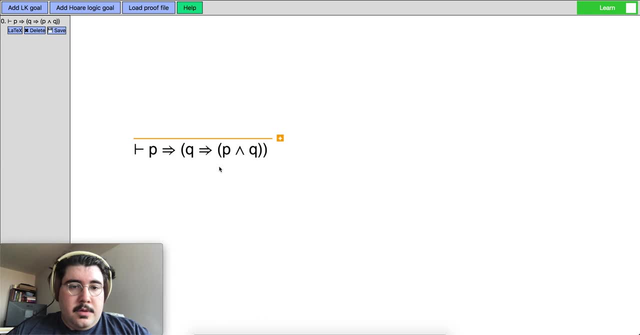 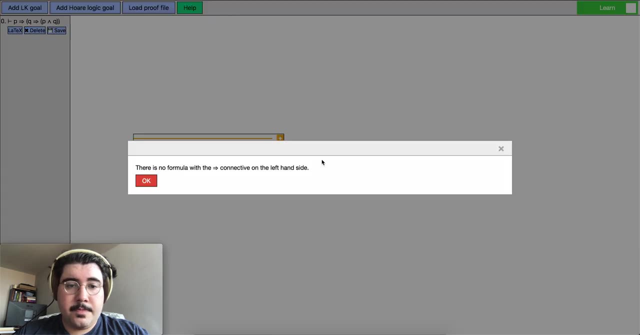 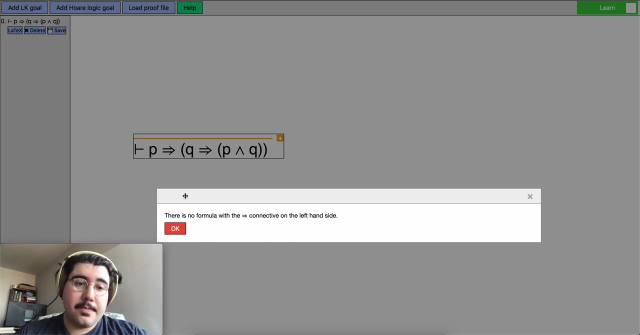 that we get for these things. So suppose we were here And instead of clicking the right implies rule, we clicked on the left implies rule And we get an error that says: you know, there's no formula with the implies connected on the left-hand side. 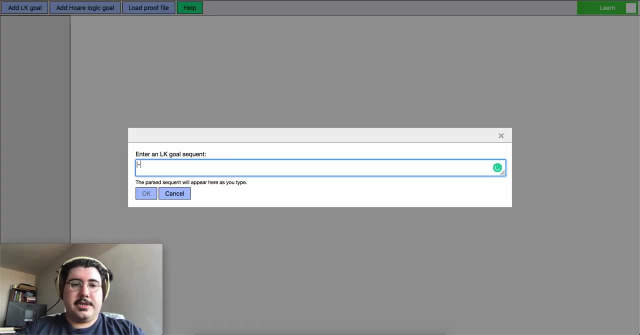 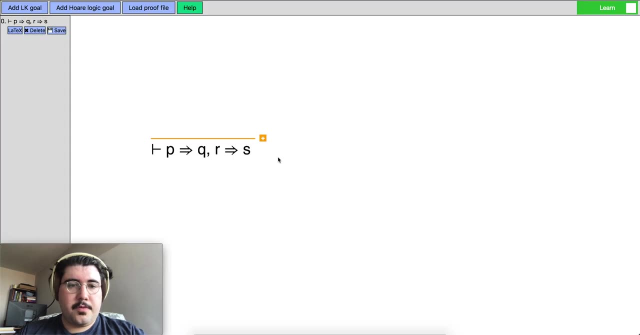 Or if we had a different rule, a different kind of goal, such as a P implies Q or R implies S. It's not provable, but we can write, we can try to prove it. So suppose we want to apply the right implies rule for this. 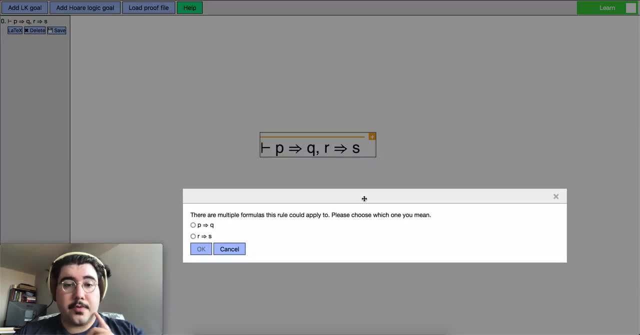 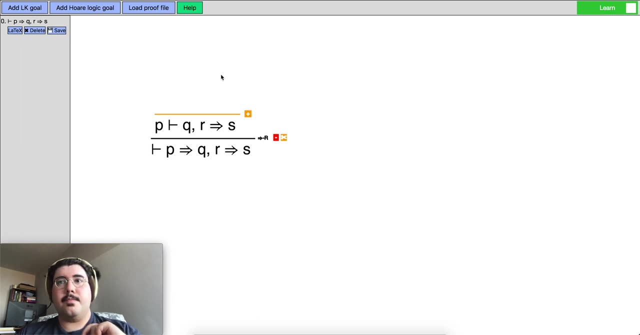 And for this one you get a question, a prompt form from the proof instance, which is like: which rule do you want to apply this on? So you can pick one and you can move on, Or if you have a goal with quantifiers in it. 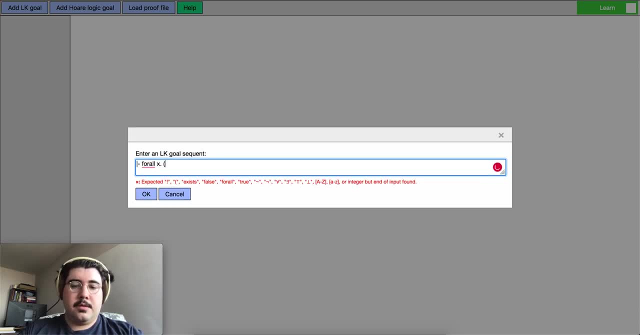 suppose you want to say for all X, or let me. let me not put this in for now, so I can show you something. PX implies PX. It's obvious. But notice how, when it parses here, it is parsing this part as 1.. 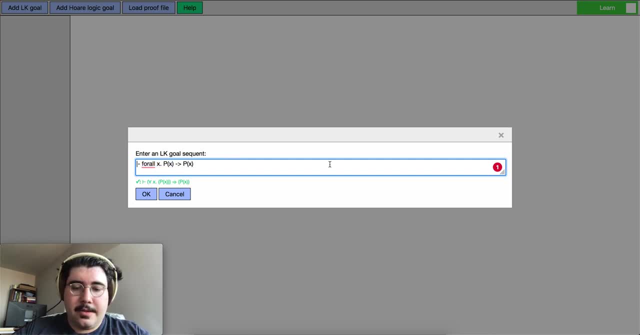 But we don't want that. So we can see the output here and we can add the X or P. So we're going to do that. We're going to do the parentheses that we need. So now, this is what we want. Okay, 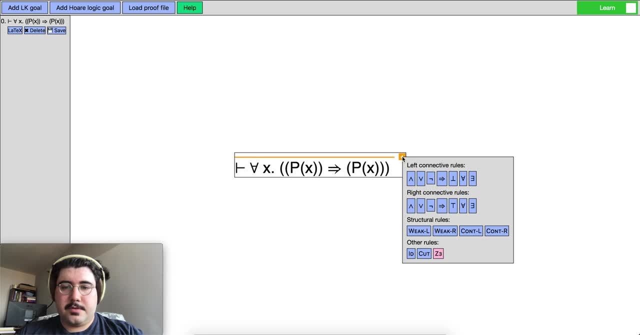 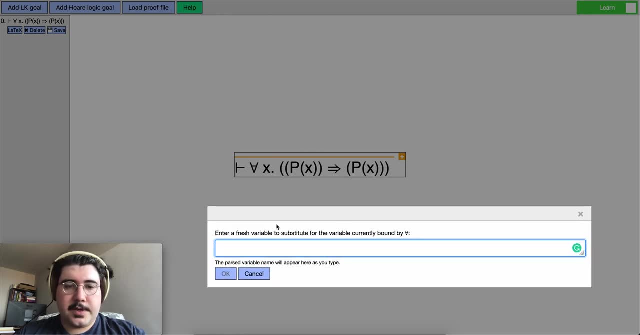 So now this is something with quantifiers, And if I want to start proving this, I have to click on the rights for all rule, And this rule says: enter a fresh variable to substitute for the variable currently bound by the for all quantifier. 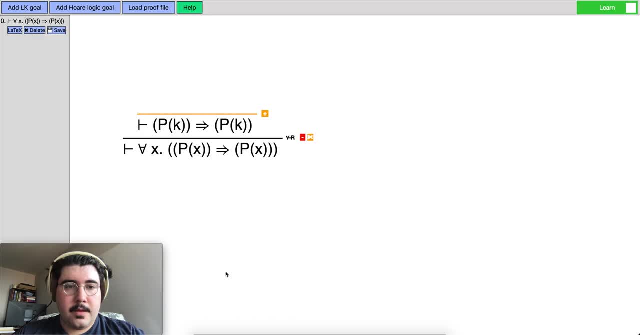 Um, we can just say K, whatever, and we get what we want. So so with X or prompts, whenever The proof assistant needs extra information about which formula to apply rules on or which quantifier, like how quantifier should be um, should we transformed? 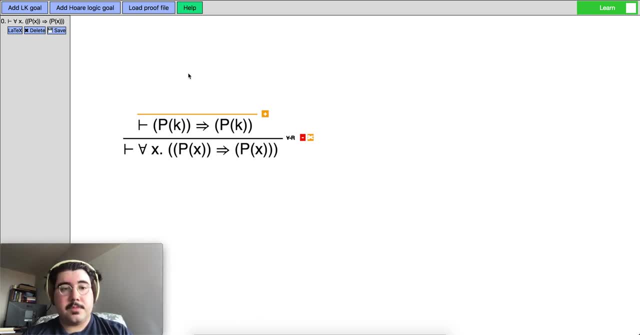 Uh, it gives you prompts and you um enter the extra information to to keep going with the proof. Um, okay, So I also want to show a different feature of the proof: tree builder. So, as you can see on the top right, 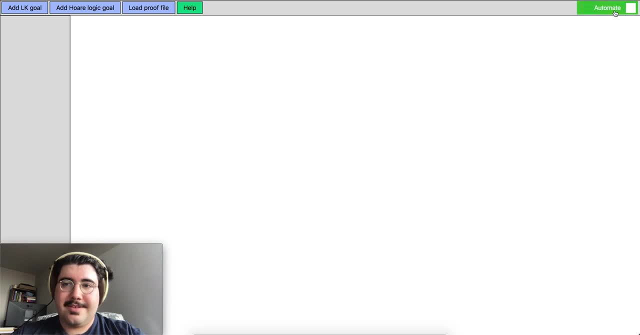 Um, on the left side we have this button that toggles between learn and automate. This is because the proof tree builder comes in two modes: the learn mode and the automate mode. Um, you want to learn mode, when? um, you are learning which rule should be applied when? and in the automate mode. 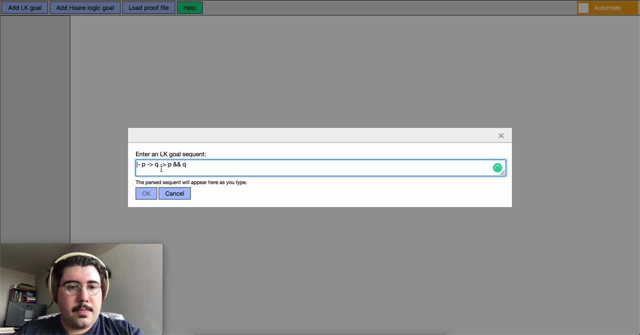 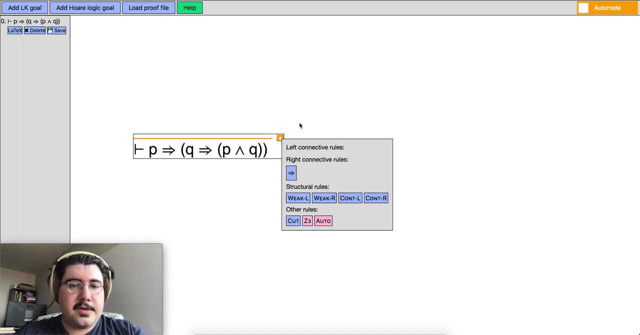 Let's go back to this example again. In the automate mode, when you click on the plus button, Uh, you don't see the rules anymore. You only see the rules that are relevant In fact. let's go back and see this again. 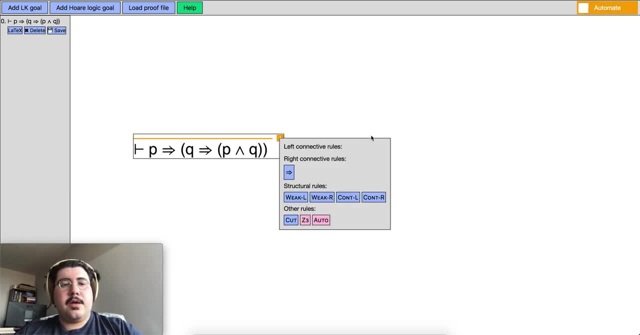 See, you have more rules. So so here, um, you can kind of tell from what formulas you have on on which sides, um which rules you can really apply Um, and this is sort of uh obvious to follow at this point, or in the automate mode, you also have this extra button called auto uh, which does 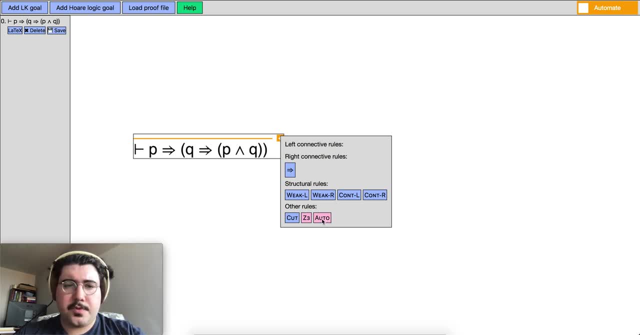 A simple proof search. It's not very clever, It just puts force in in certain ways and it stops when it has, when it has some kind of ambiguity about which way to go in the proof. But for this simple example it can prove automatically. 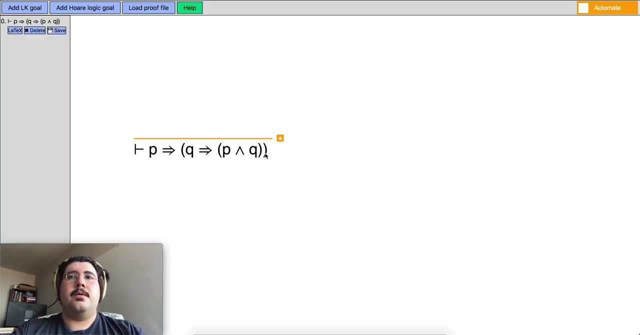 Um, okay, So I also want to show you a horologic proof. Okay, Now suppose you want to prove the horologic goal for a simple program. So I click on the add horologic button and then it asked me to enter a whole triple. to suppose I want to prove a simple program. 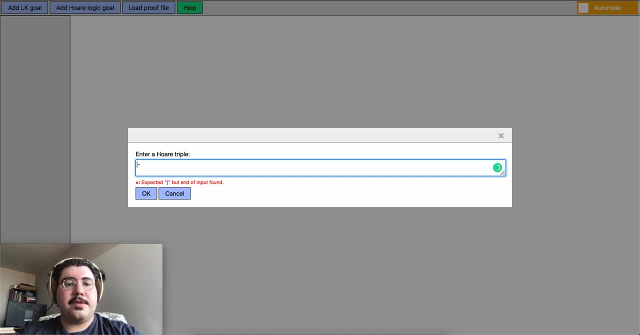 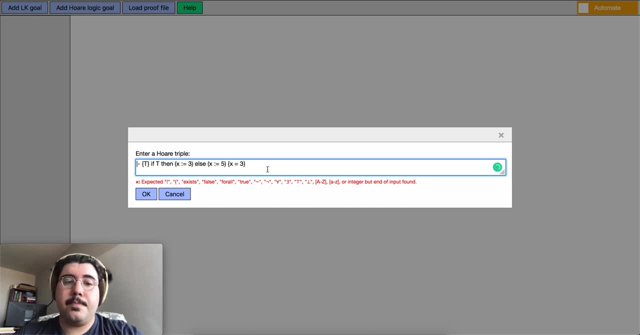 Okay, Okay, Okay. And of the as a as a post condition, and we say X is equal to 3.. So, just by, by the fact that the, the conditional here, uh, the condition of of the statements being true or truth, um, we should know that X ends up being three. 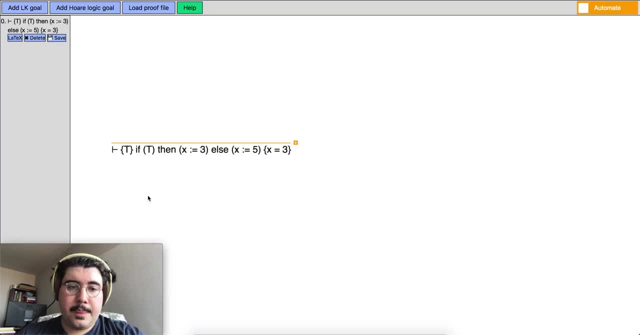 So I press an And then I get my incomplete proof tree. Okay, And then I get my incomplete proof tree, So I want to proceed with the proof. I click on the plus button so I can apply the condition conditional role, or I can apply the mean to the particular condition level. 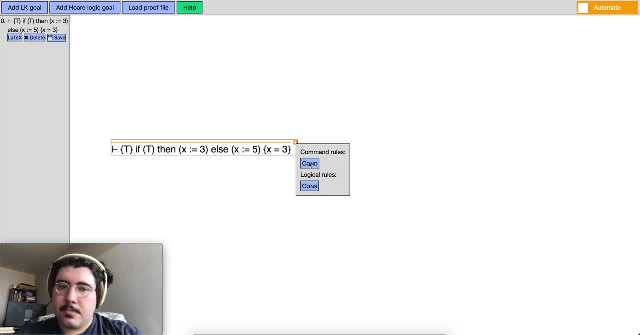 So, uh, can you see what's going on with that? or I can apply the consequence rule, so let's apply the conditional rule. and then we have multiple subtrees. so now the rule for the assignment. so when I click, I get the assignment rule and the consequence rule. the rule for the assignment requires the left side to look similar. 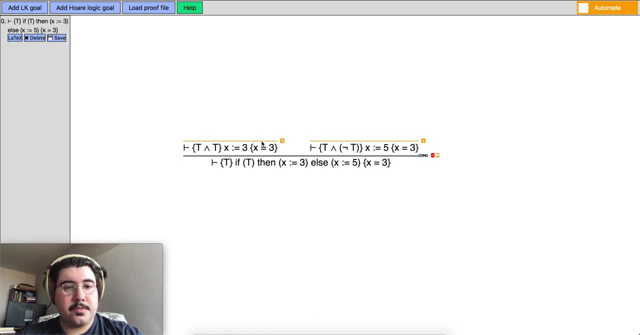 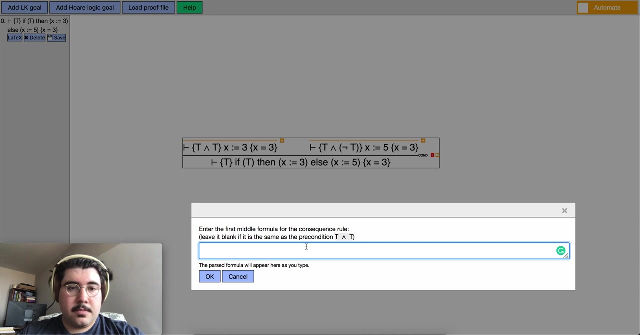 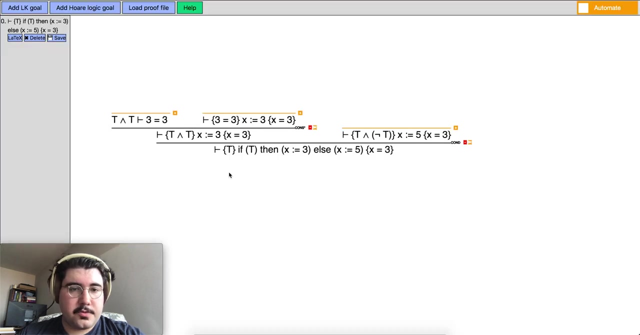 to the right side in certain ways, and then we're going to substitute one thing to get the right left side. so for that I had to put, I had to apply a consequence rule. so I say, suppose this is just 3 equals 3, and then we don't need the second formula for the consequence rule. this is a proof. 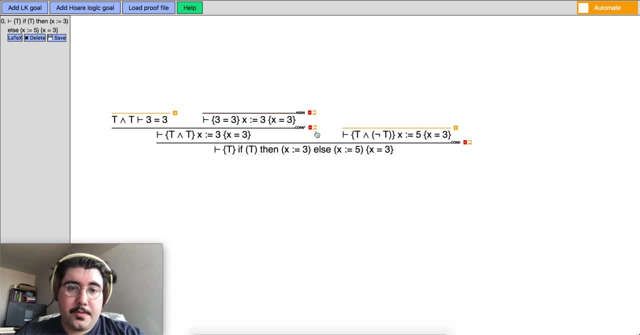 street that we get and not here, we can apply the assignment rule. I'll get back to that later. so on the right side of this big burst tree we have another assignment statement, and here I well, here, when this on the precondition we have truth and not truth. so we can, we can give. 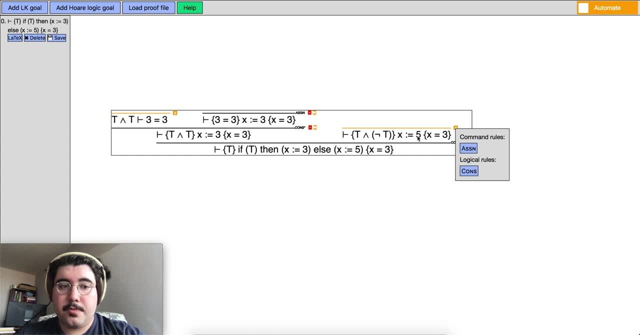 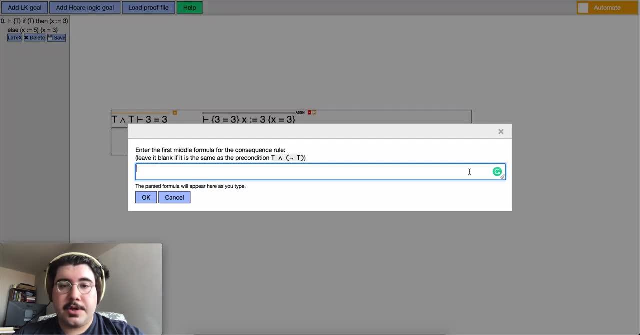 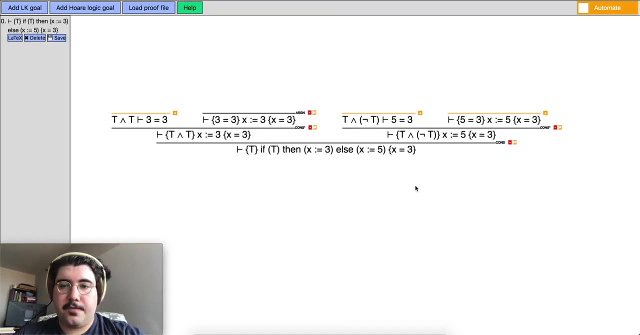 whatever kind of formula we need to get the assignment rule going and then we can just discharge the proof on the left side. so another consequence rule application here, and here I want to say: 5 equals 3, so here I can just apply the assignment rule again, and that's good. so now what we have here, as if you. 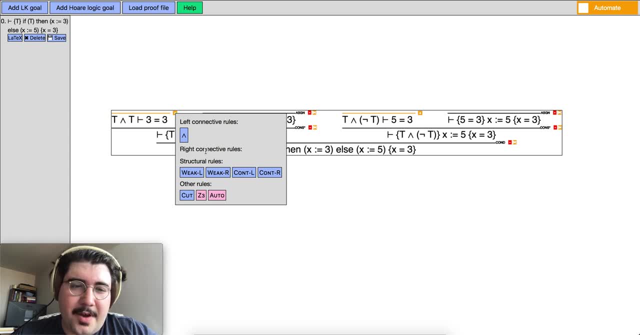 press plus you see left connected rules and right connected rules and structural sequence calculus rules. so this is actually the whole reason behind this proof assistant, because inside horologic proofs you may need to do sequence calculus proofs and our system by calling it according to what we call parins' rules- and, by the way, part 2 proves that proof is random in obj. 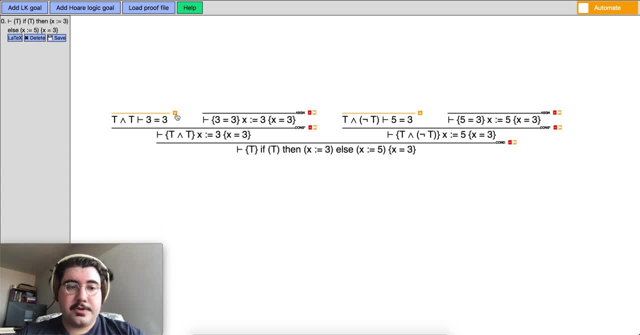 and says: I have now created a set of vanishing exist sentences and the things, the sentence that comes to mind as it relates to these SQL Bye color via them to broth rules. So now we would think, if I do this again, I would be Carr platon. 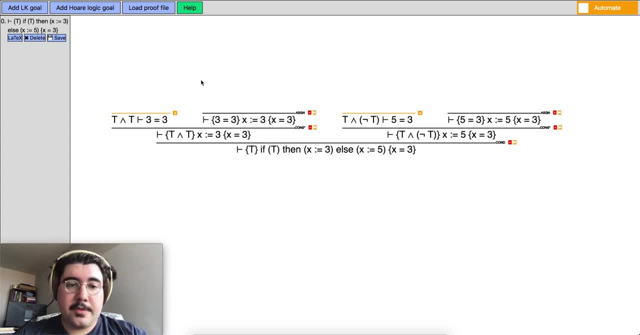 altogether. I would have just using the proof rules that we have. we cannot discharge this rule. and also, if you're writing a horologic proof, most of the time this part is not what you're interested in. so we added this feature using z3, that when you press it. 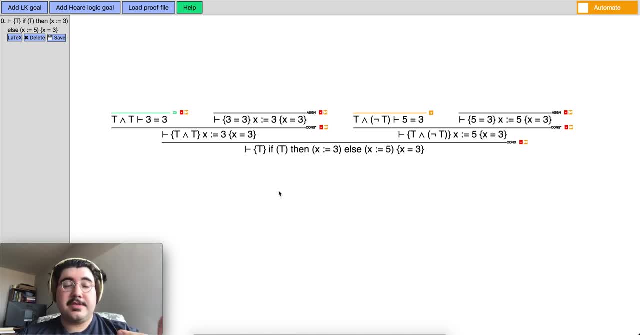 it generates an smplib file and runs that, runs that in z3. so there is a version of z3 compiled to WebAssembly using Emscripten. it is currently about 19 megabytes or so. that is actually loaded in browser, but we can just run it inside our browser like this, just on the client. 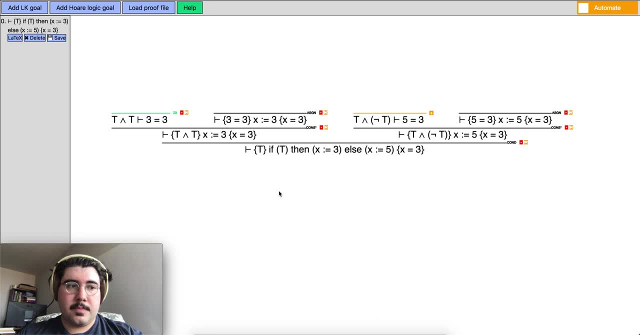 side. there is no server, there's no service side communication about your proof goals. uh, we can do the same thing for the other. uh proof tree here and that also says green. so notice how, if the goal, um, if if z3 finds your goal to be valid, 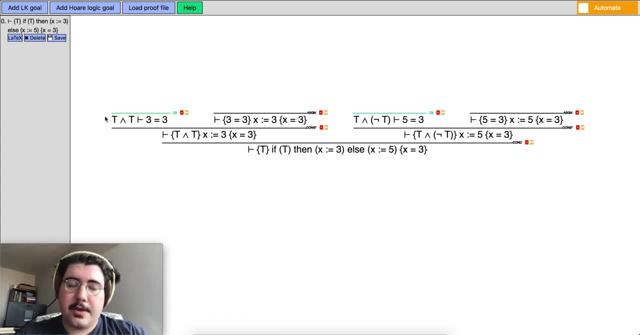 then we put a yellow- sorry, a green- line over your proof. so this is sort of meant to be sort of a pseudo axiom, as i call it, not a real axiom. like users know that this is not a real proof tree, uh, but this is not something we care about proving right now, but we just want to check. 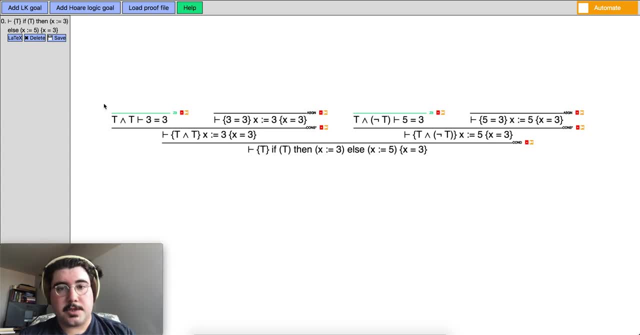 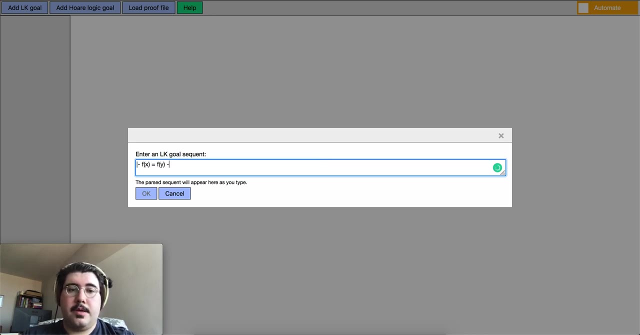 it, if it's correct, uh, using other automated reasoning tools, and that's that's what we use this feature for. i also want to show you a different use case of the z3 rule. suppose the user wants to prove a goal like f of x equals f of y implies x equals y. so for any particular goal, 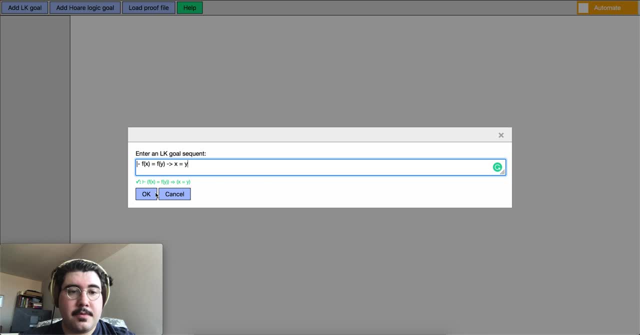 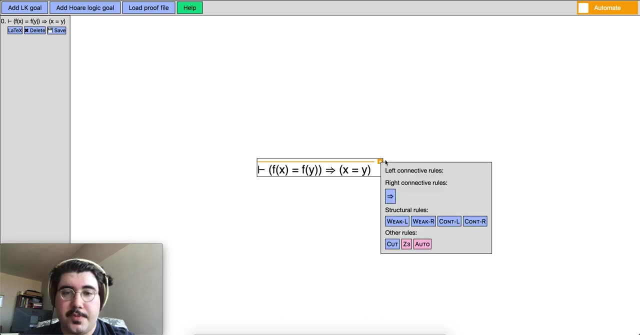 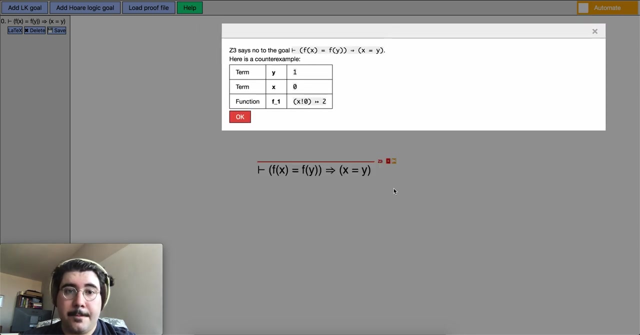 f, x or y. f is injective, So we know that this is unprovable. but if we try to prove this, if we press plus and then z3, we are gonna get this, this prompt back. It's gonna say z3 says no to the goal and also puts a red line over.